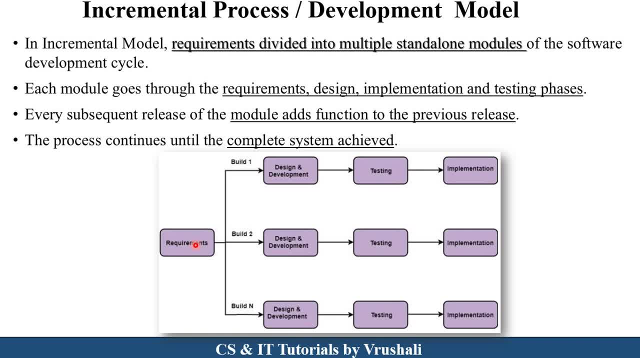 the customer After collecting requirement. they divide the requirement into the multiple module as per the priority of customer. Suppose customer want first priority attendance module. Now they build attendance module. They design, develop and test implement attendance module. Now the second one is student feedback module. So they design, develop, test and implement student feedback module. And now the third module is class test module. Now they design, develop, test and implement student feedback module. 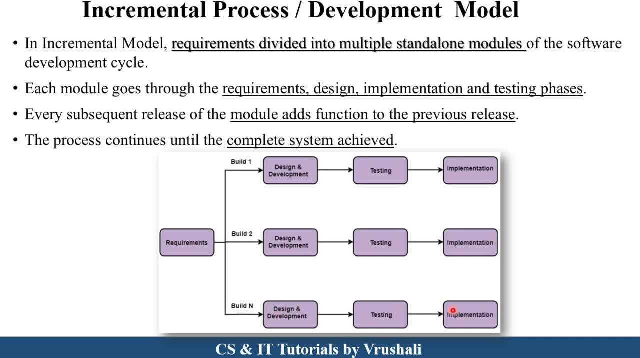 Now the design, develop, test and implement class test module in this way. Basically, every module is goes to the complete software development lifecycle phases. like design, develop, testing in this way Clear. So this is a concept of incremental process model. 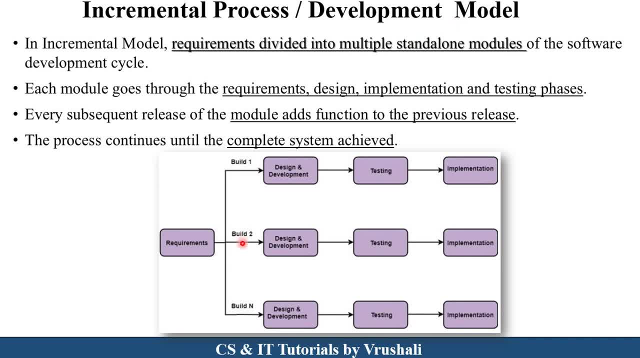 They develop a particular product or they develop a particular project module by module, not a complete project at the same time. First they develop first module, that is, attendance module, and they deliver this module to the customer. After that they develop student feedback module. 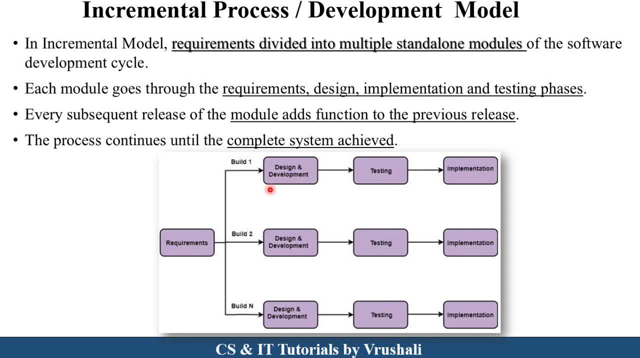 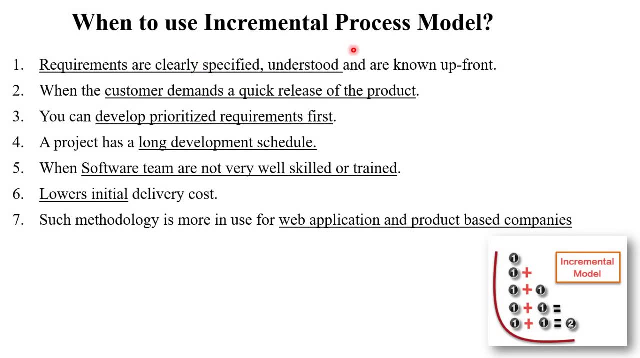 Again, they deliver this module to the customer in this way. So, after completing all this process, at the end complete product was developed. So this is a concept of incremental process model. Next Now, when to use incremental process model. So, as we discussed the concept of 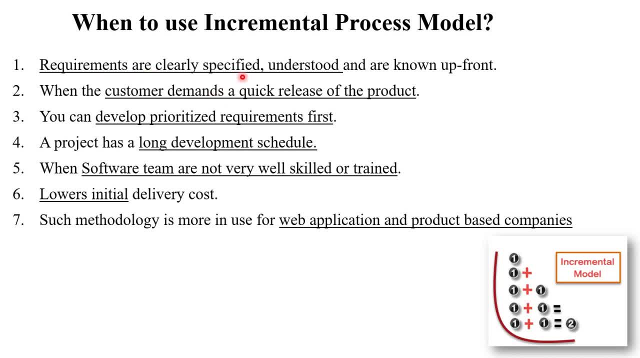 Incremental process model. here customer requirements are clearly understood and clearly specified. Customer know that, what type of features and what type of models they want in their particular project and which type of priority model right. The next thing is when the customer demands for quick release of product. when customer quickly want a particular product or particular model. 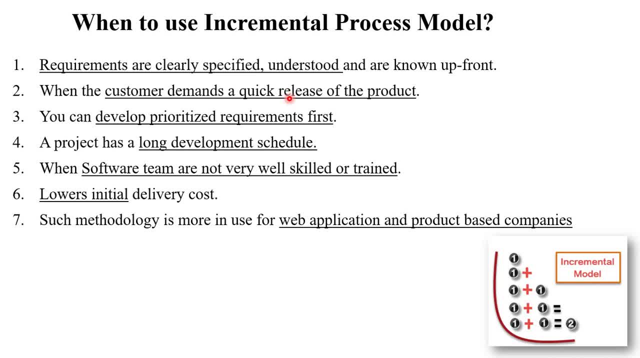 Suppose a particular organization. They want attendance module First, So there is a quickly release of that particular model. Now the next thing is: a project has long development schedule. Suppose a particular product, for example college management system. They want multiple modules again, like alumina module, then training and placement module. in this way: 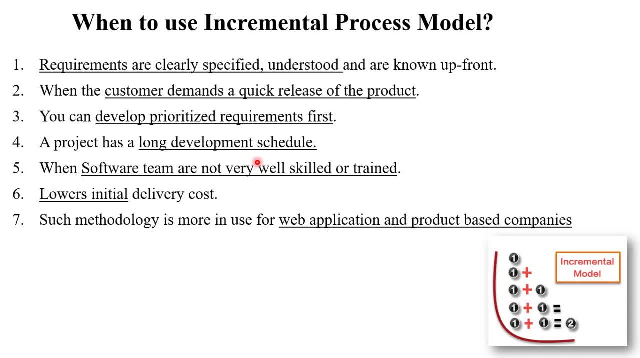 So this is a long-going project, not a short project, right? So incremental process model used for long development project. Okay, The next thing is here: Software team are not very skill or train because you need to develop a project module by module. 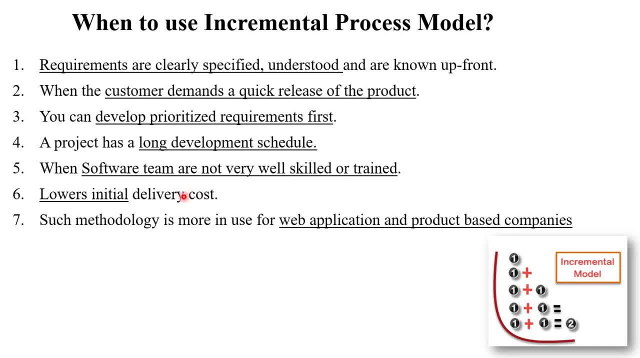 Every module has their own cost here. Okay, Suppose attendance model first developed, So developer team got their cost of attendance model after that next model in this way. So generally this incremental process model used in different web application and different product based companies where different Android apps than websites have developed. 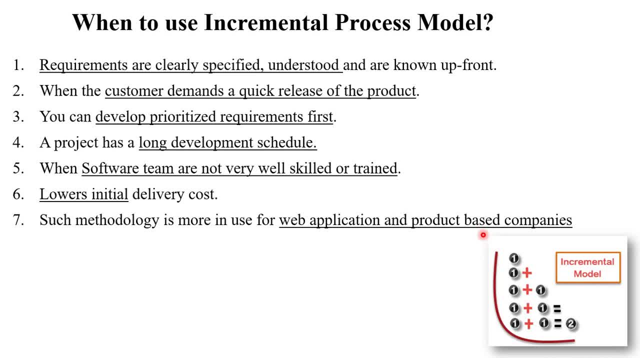 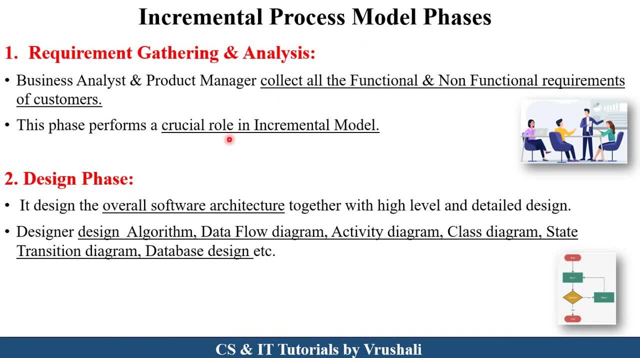 Where incremental process model have used next. Next one is incremental process model phases as we discuss software development life cycle. The first phase is requirement gathering analysis. Here business analyst or product manager collect all the requirements, like functional and non-functional requirements, from the customer. functional requirement include what is the need of customer? 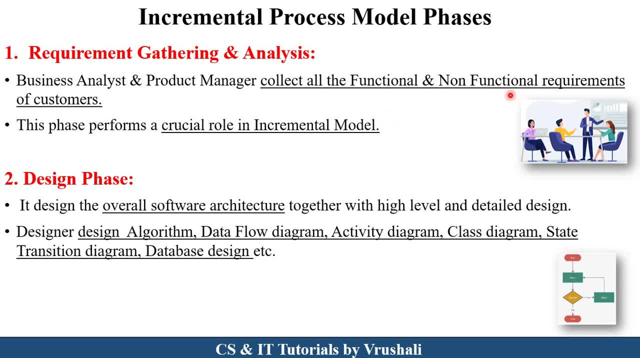 What exactly customer want, and non-functional. The requirement means how your product look like in future. So in incremental process, model requirement gathering play a very important role. Okay, because everything, every module has based on the requirement or priority of requirement. The next phase, design phase. after collecting all the requirements, designer team design a software architecture means how your product look like in future. 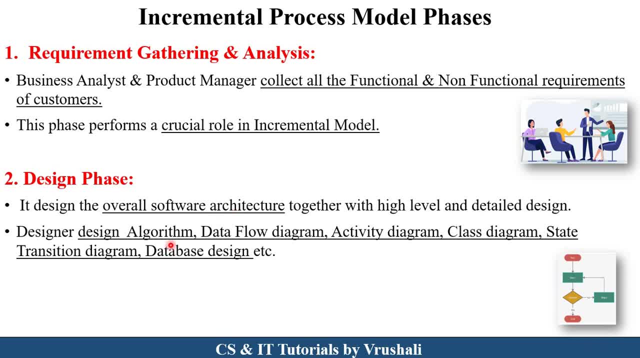 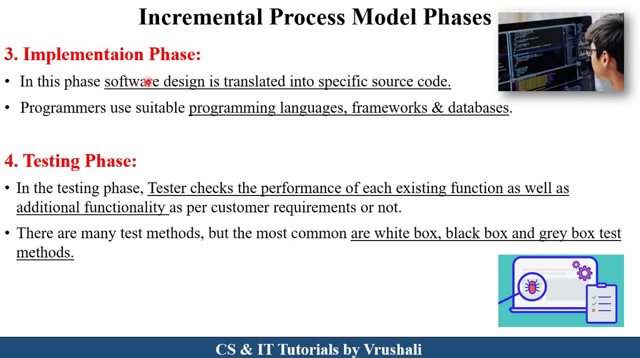 They design a particular product. for that purpose They design algorithm, The data flow diagram, activity diagram, then class diagram, database design, Etc. Next, after designing a particular product, the next phase is implementation phase. here programmer develop a particular product by using a particular programming languages for that purpose. 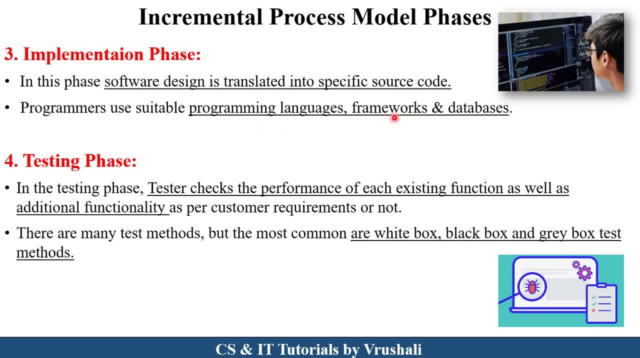 Programmer use different source code, different frameworks or different databases. Next one is a testing phase. after developing A particular product, tester check the performance of each and every model. every model is as per the customer requirements or not. So this is the work of the tester. for that purpose, 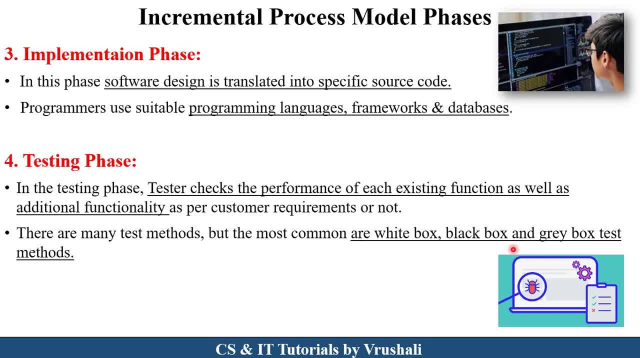 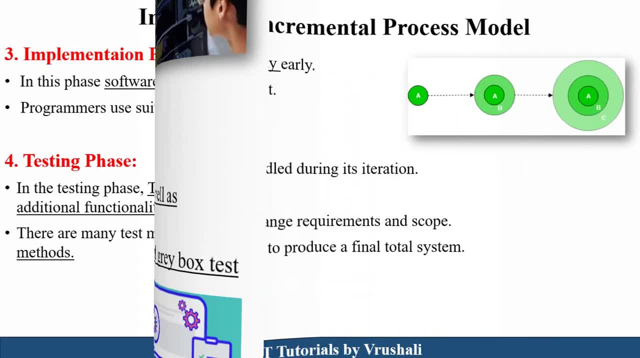 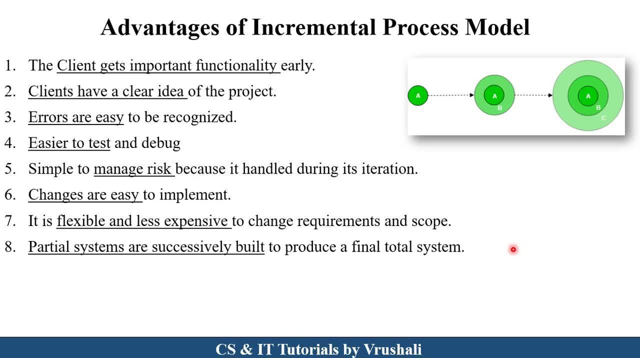 They use different testing methods, like white box, black box. again, There are different types of testing methods that will be suitable for your product next. So, after testing of each and every model, they deploy the particular model to the customer. now, Advantages of incremental process model. the first and most important advantages is here: